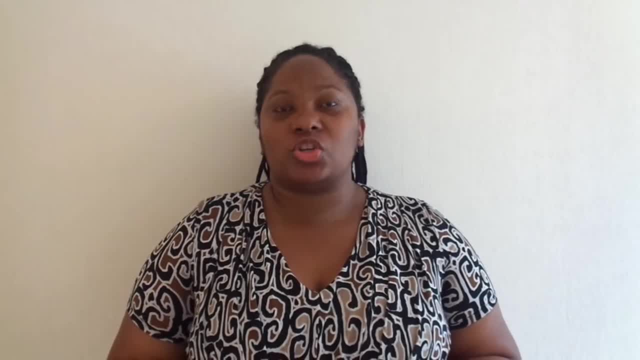 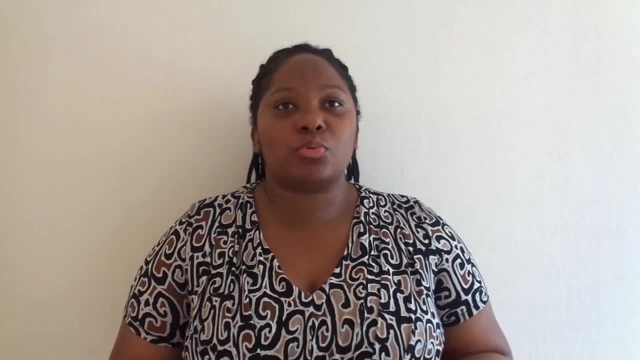 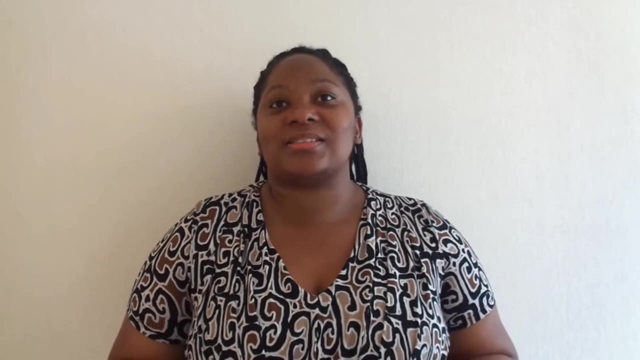 their pedagogical skills through mentoring and coaching. This means spending time solving pedagogical problems and improving their teaching skills. Instructional leadership also requires problems taking actions to improve teachers' methodology and holding teachers accountable for improving their modelling skills in a supported system. 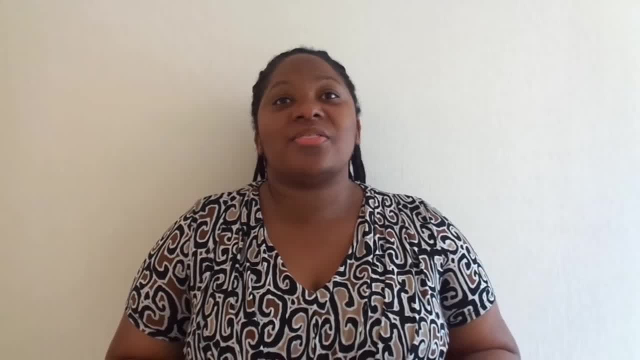 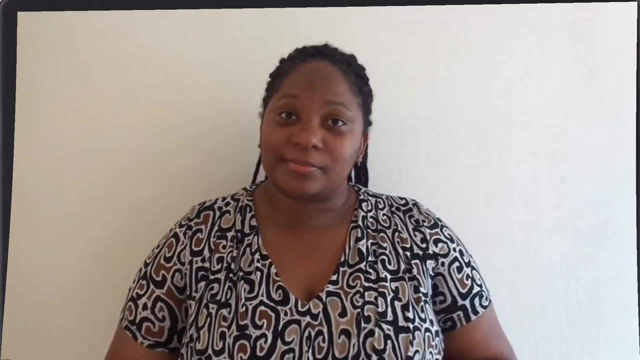 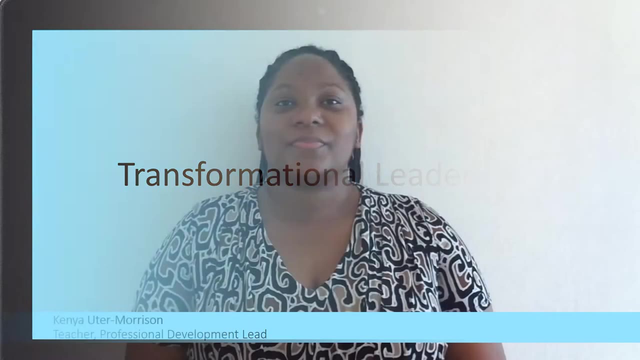 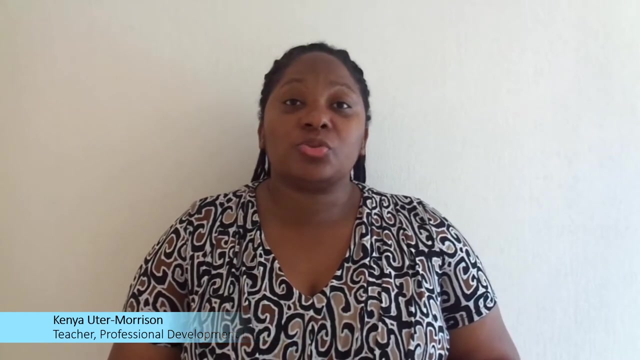 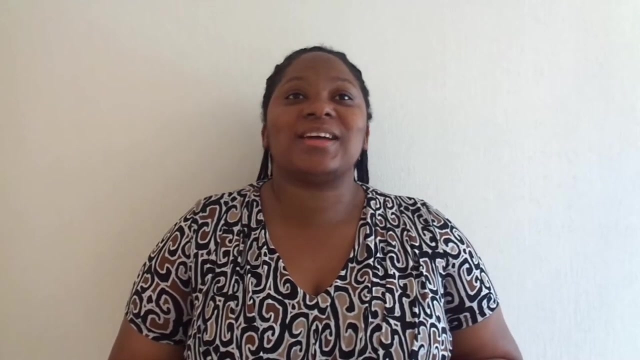 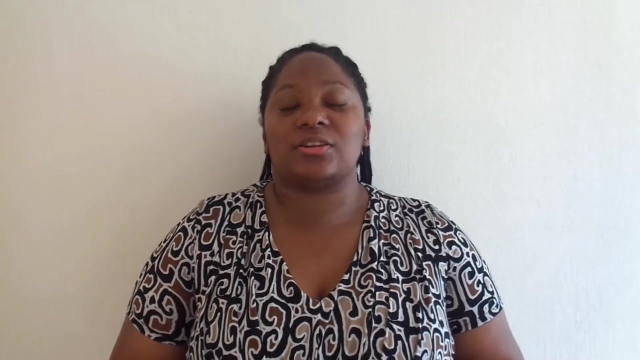 Teachers in their classroom also need to use this leadership strategy in supporting students' learning and achievement. Transformational leadership is a productive relationship style which uses individualized consideration, inspirational motivation, intellectual stimulation and idealized influence to develop people. It takes the form of individual support to instill trust, admiration and respect, which 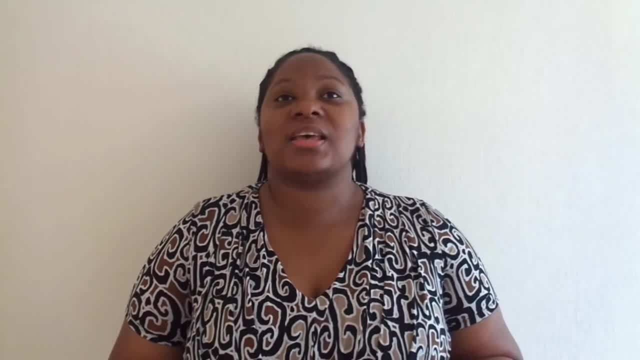 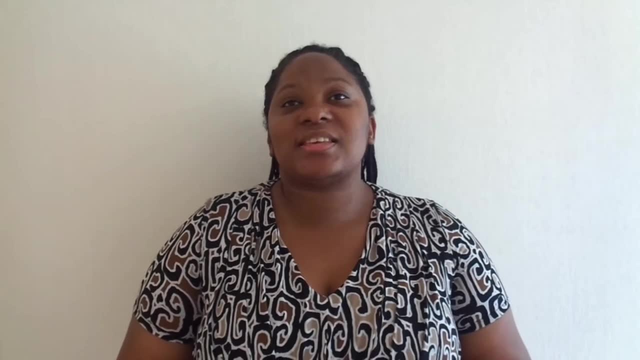 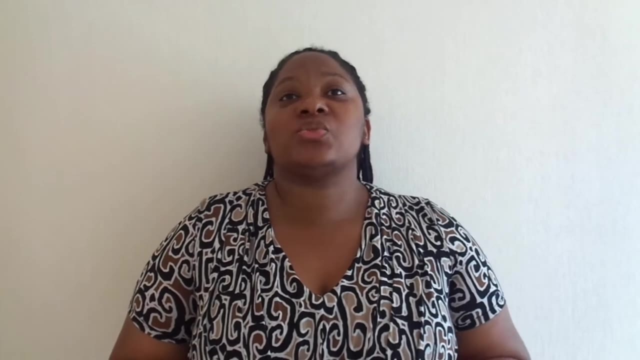 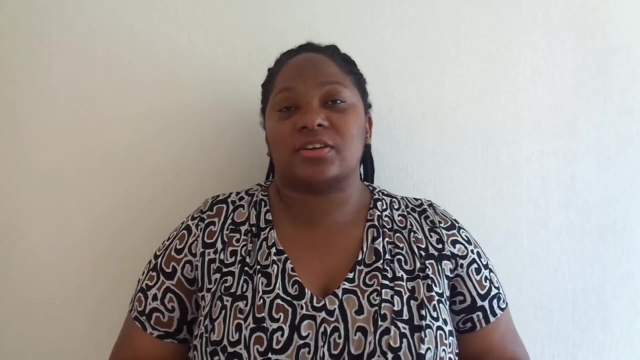 by extension, inspires, motivates and improves morale and advance performance. Transformational leaders possess the skill sets required to monitor and manage their own emotions and thinking as well as those of others. This gives the ability to energize teams and drive successes When students or staff are encouraged, inspired and motivated. 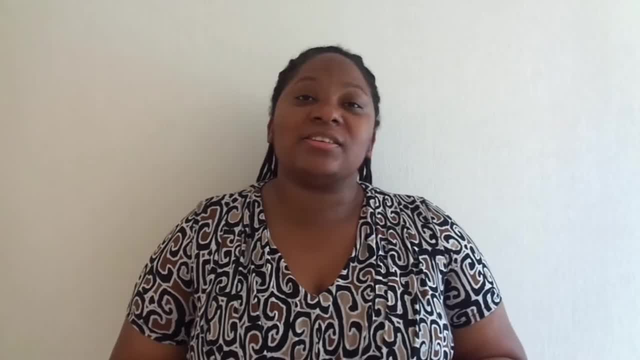 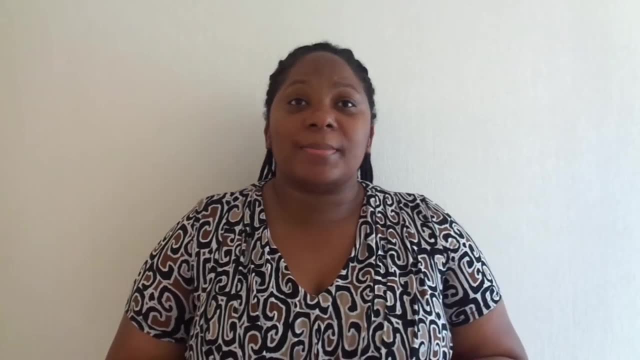 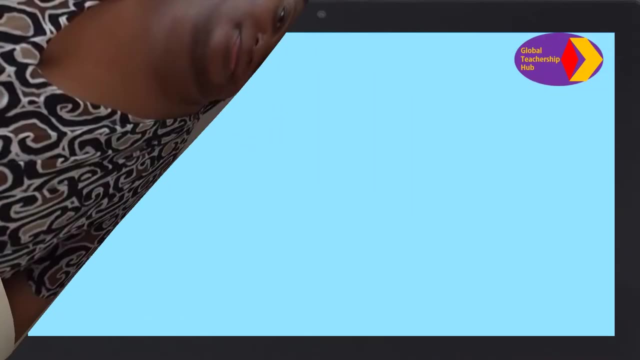 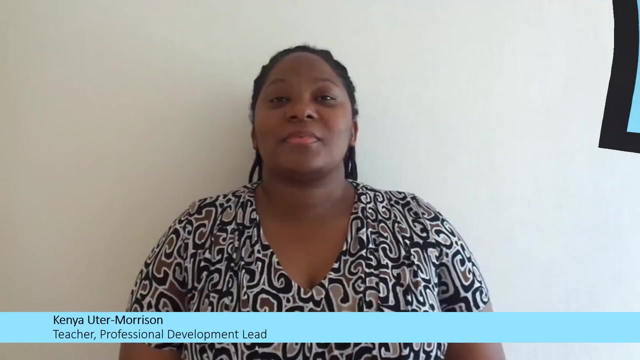 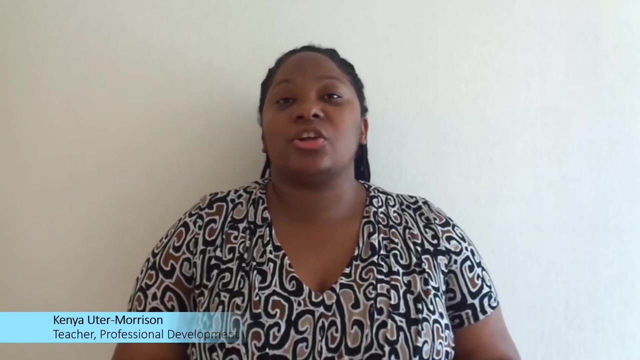 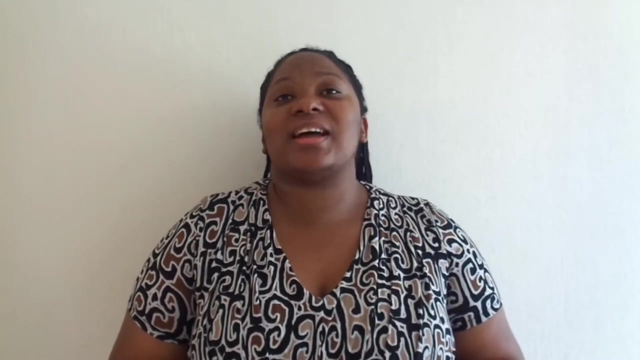 they are better able to innovate and create change that will help grow and shape future successes. These transformations result in longer lasting progress across the school community. Constructivist leadership aims at facilitating diversity and inclusion and learning rather than dictating. It involves immersing teachers and students in a culture of 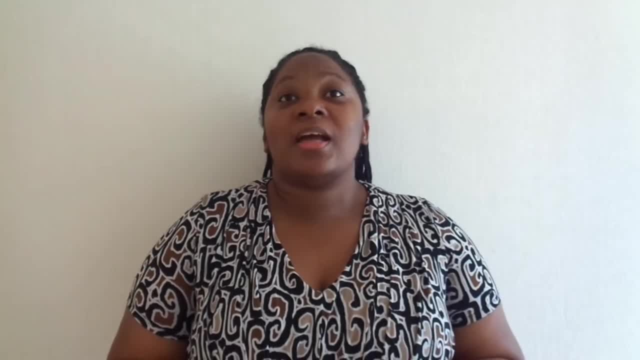 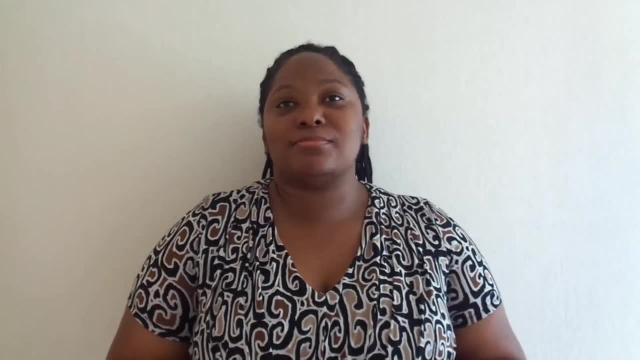 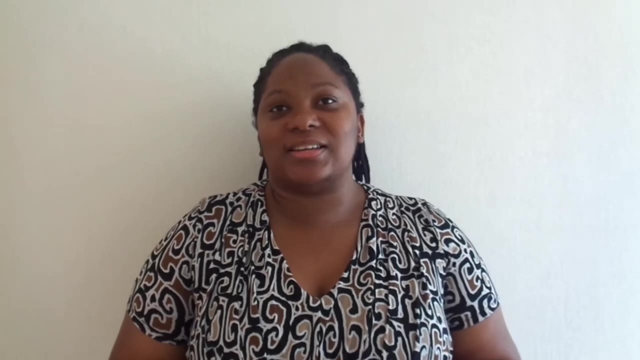 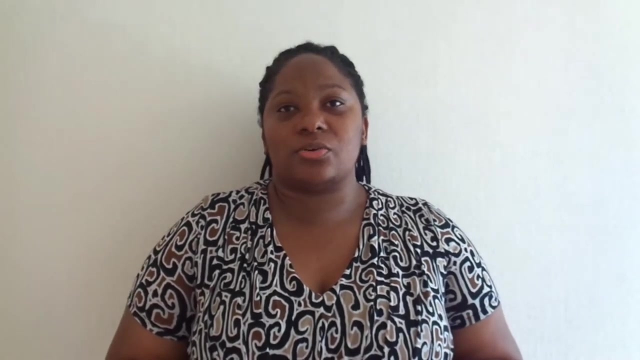 learning and enabling them to take risks. This is off the back of acknowledging that every learner understands processes and gives meaning to learning through their own realities. Such approaches allows teachers and leaders to place a priority on customizing teaching approaches that takes into consideration individual learning and developmental needs. 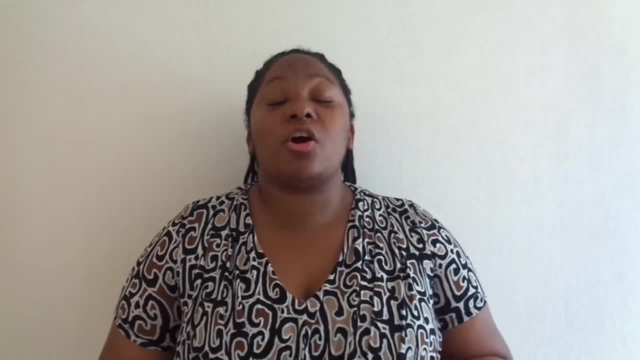 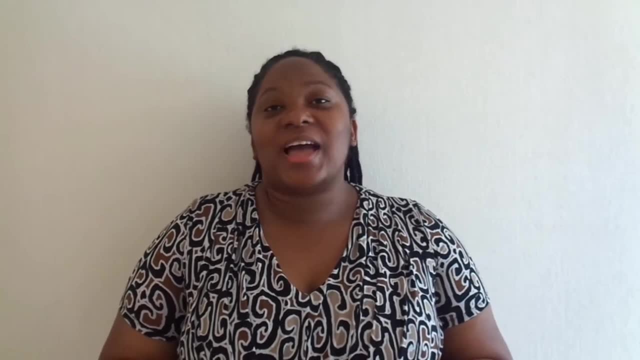 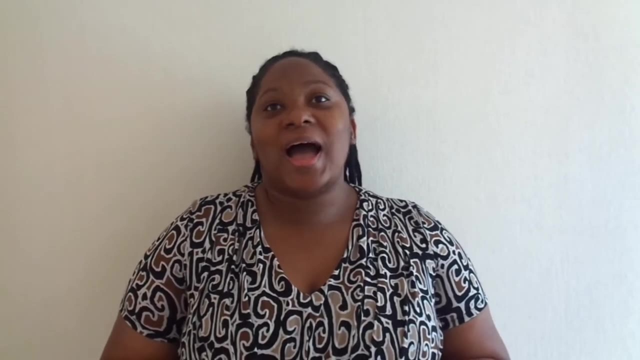 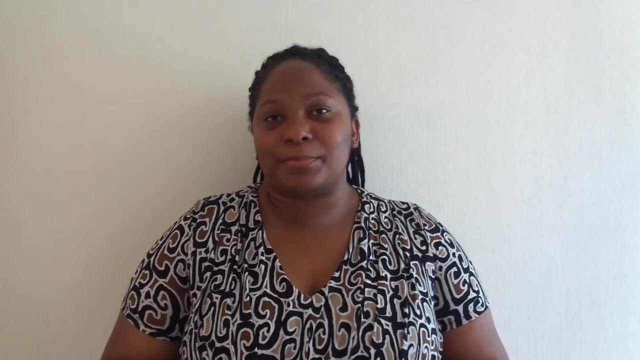 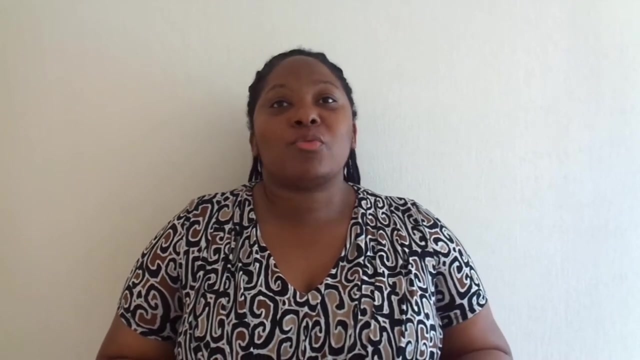 Constructivist leaders encourage the sharing of big ideas and challenging others' perspectives. They expect, facilitate and encourage teachers' engagement in reflective practices and processes, personally and with their students and peers. Both a reciprocal process and spiritual concepts are evident in the constructivist leadership approach. It enables related participants to construct meaning and embrace reciprocity. 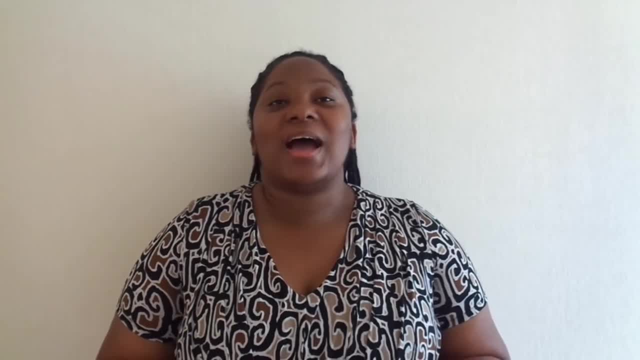 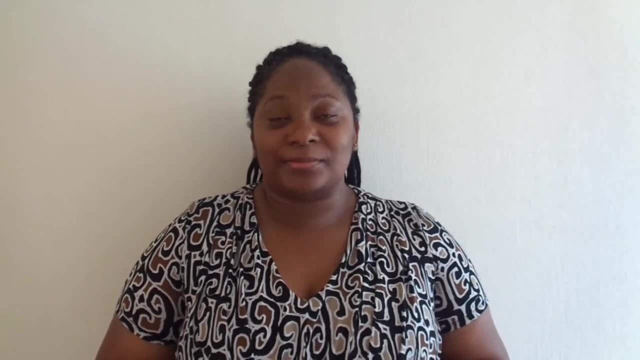 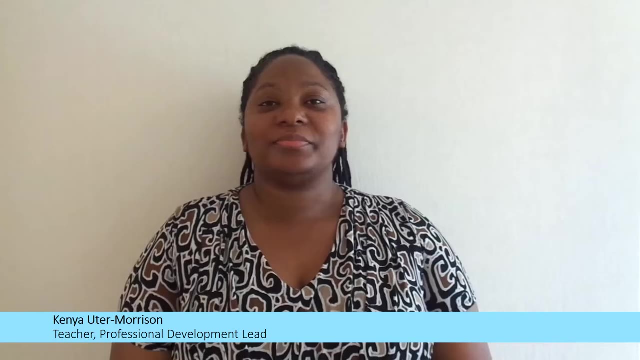 equity, learning, responsibility and community, thereby building unity and cohesion in the wider school community. For example, students must be prepared to learn from their peers and follow their experience. They must be able to share their experiences and understand their strengths and weaknesses. 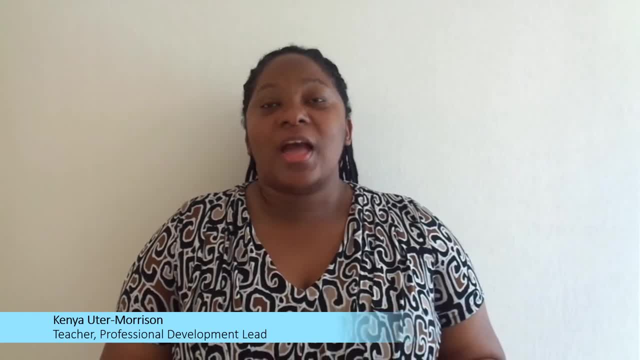 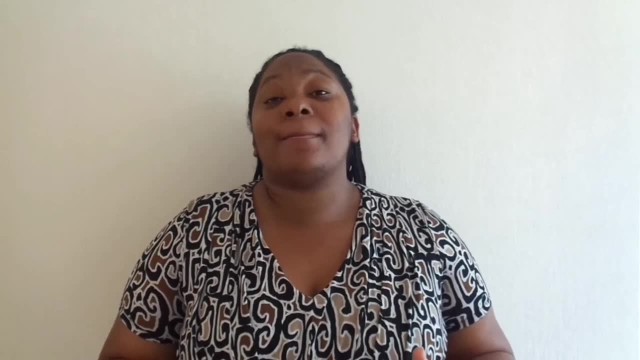 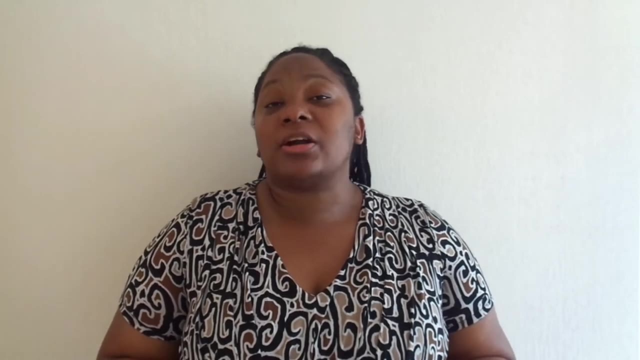 Servant leadership is built on the philosophy that the goal of a leader is to serve. These leaders instill the desire for improvement while maintaining a focus on both results and relationships. Such leadership is a participatory style which pushes ego aside and considers the need to improve. 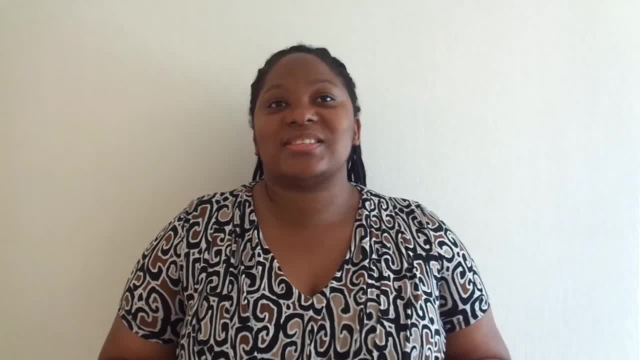 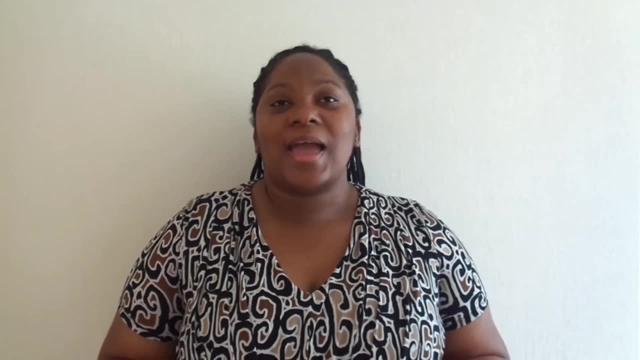 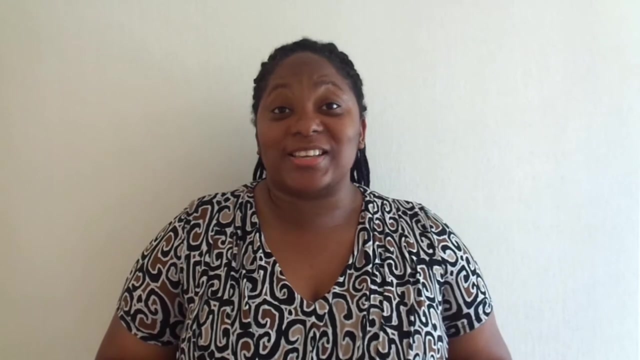 of others rather than focusing on self-interest. Some qualities synonymous with these leaders are listening, empathy, restoration, awareness, persuasion, conceptualization, foresight, stewardship, commitment to growth of people and building communities. Servant leaders shares the power of decision-making and. 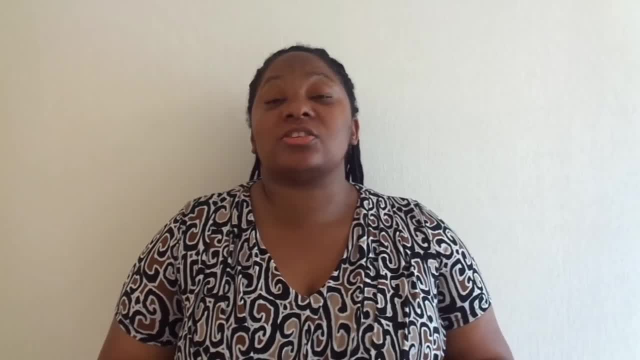 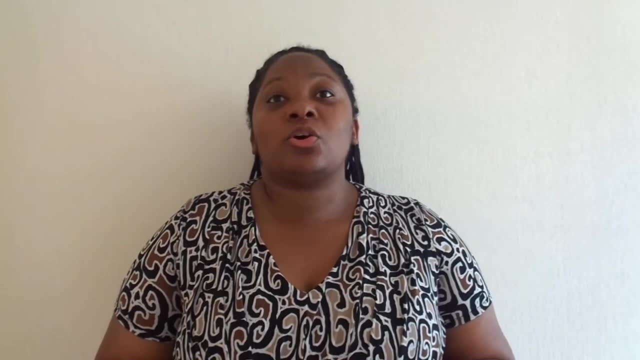 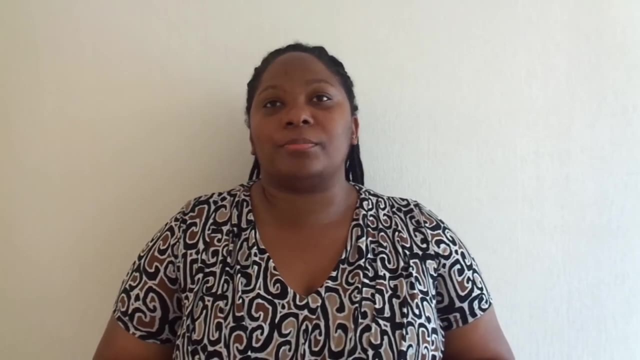 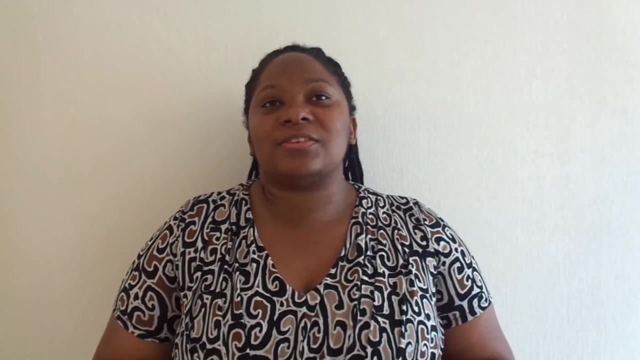 motivate and persuade their school community to fulfill their long-standing vision. This leadership style empowers the team because it puts the team members first and, at the same time, taken into consideration the overall objective and purpose of the leadership agenda. Servant leaders are able to cultivate high-performance teachers by removing 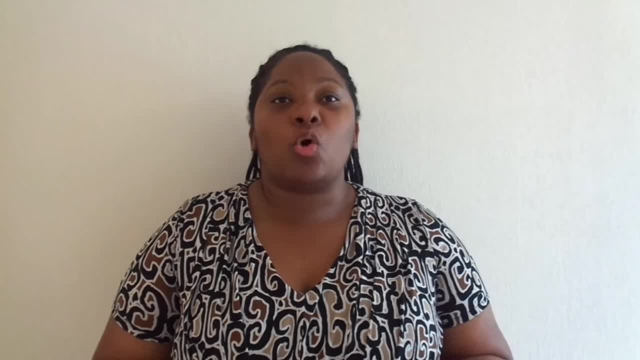 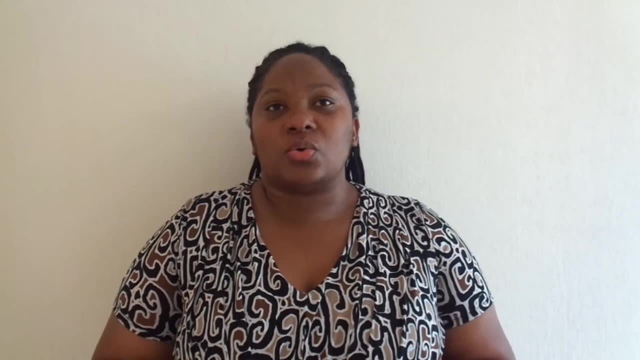 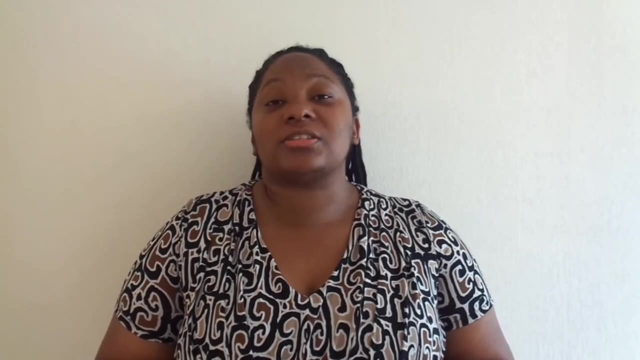 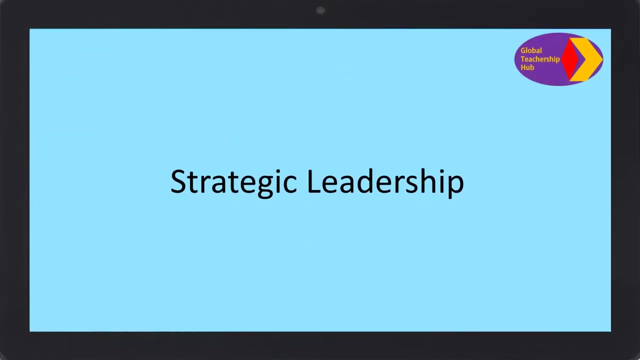 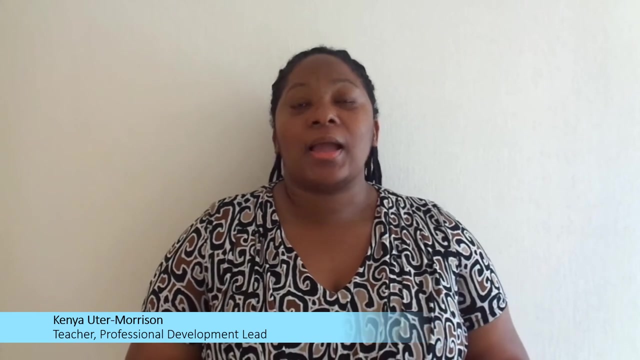 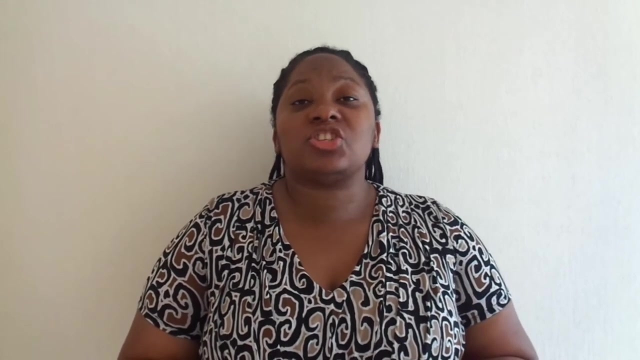 barriers, providing resources and opening communication channels. that reduces the feeling of isolation. Research shows that, in the long run, servant leaders create a positive and productive school environment. Strategic leadership is a long-term projecting, planning for future eventualities using research, data and trends Strategic leaders possess. 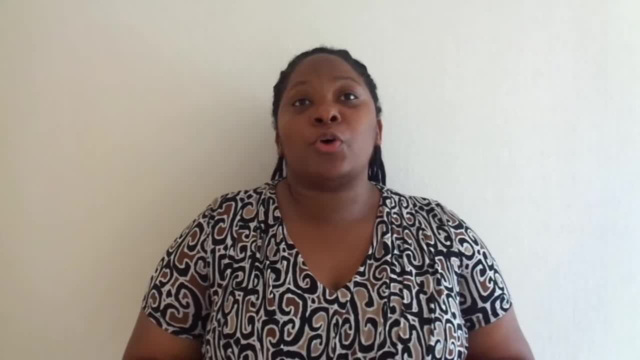 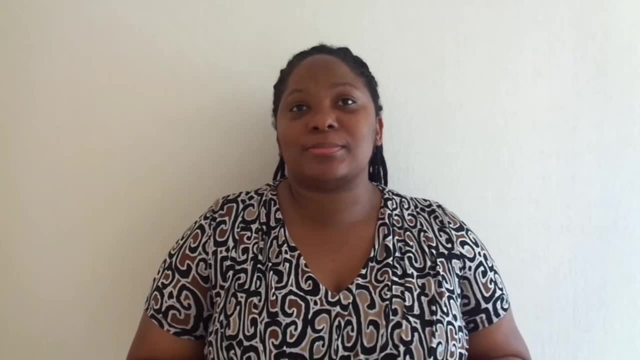 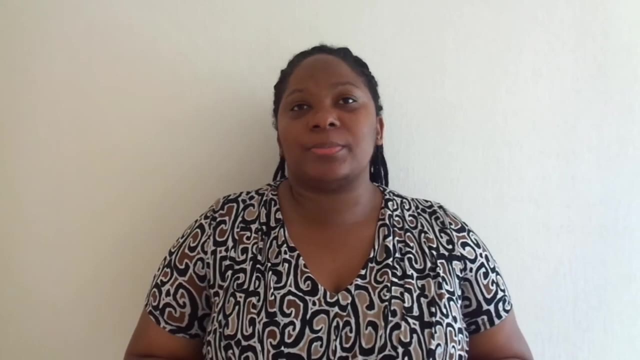 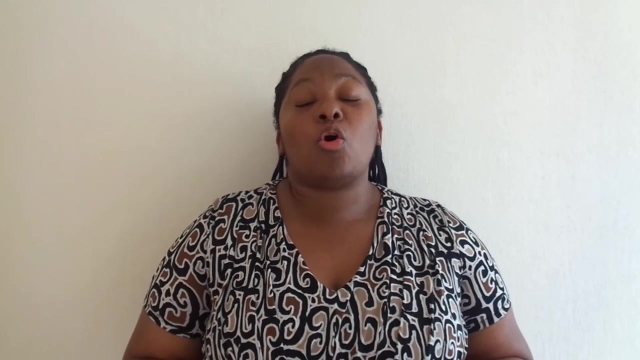 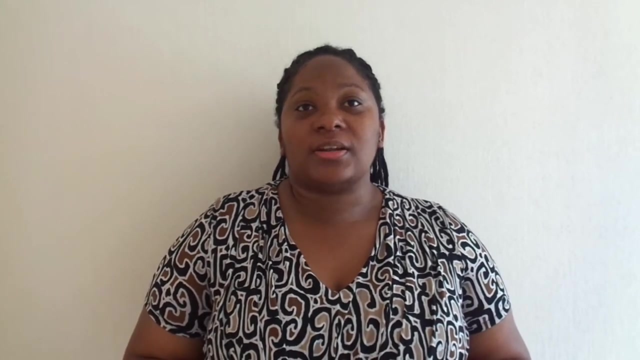 the ability to influence others, to voluntarily make decisions. that enhances the prospects for long-term success whilst maintaining short-term stability. Strategic leadersstadishهمcom will respond with the most suitable approach, whether this is staff training, reviewing policies and procedures or fostering a culture based on measured success. They use innovation and 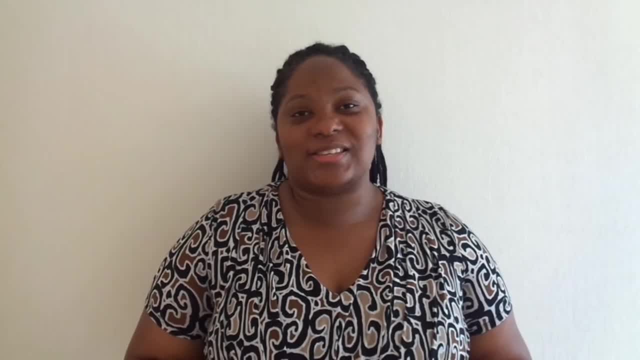 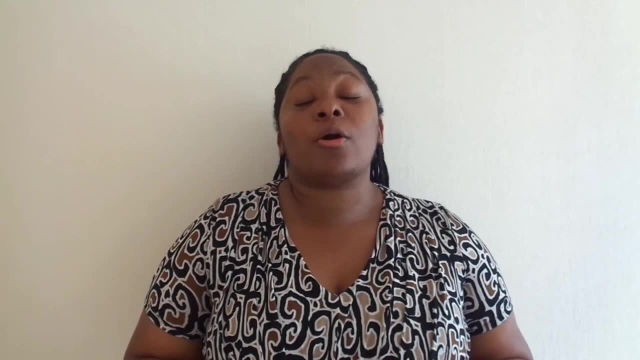 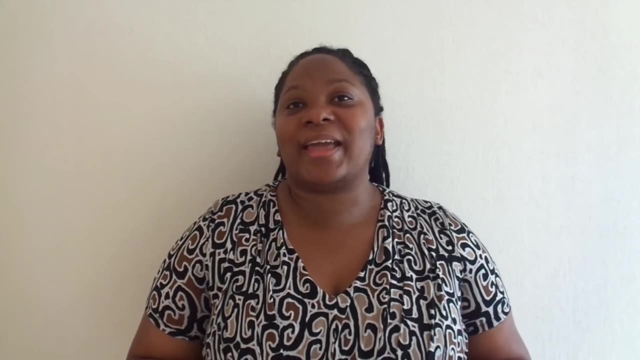 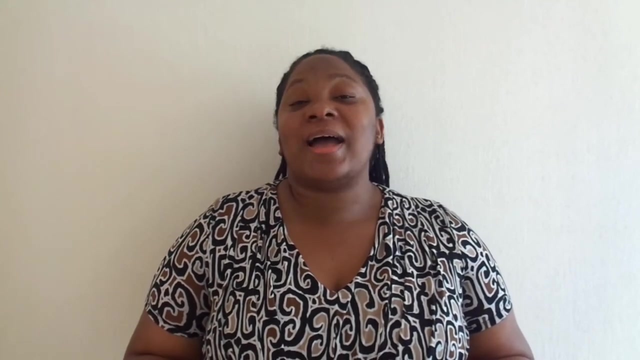 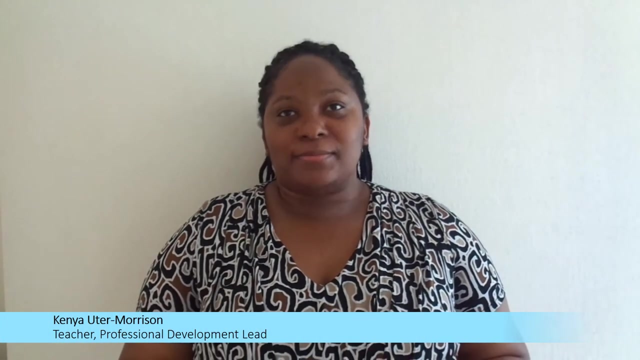 innovative thinking to improve the learning community and enhance relationship building, as well as diversity embracing or partnership creating with all stakeholders. Strategic leaders use the powers of collective thinking to build a value-based school where ethics, accountability and transparency are pillars of their leadership. Teachers and administrators need to have the wisdom to recognize the best leadership. 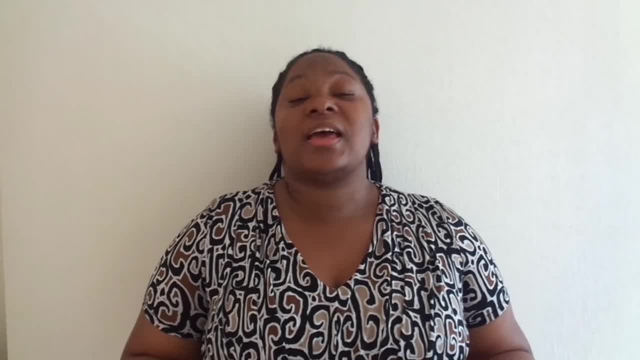 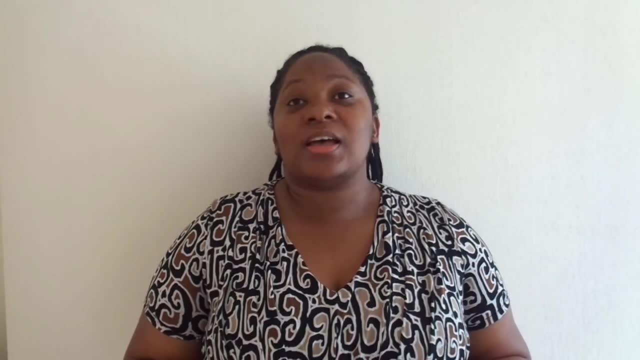 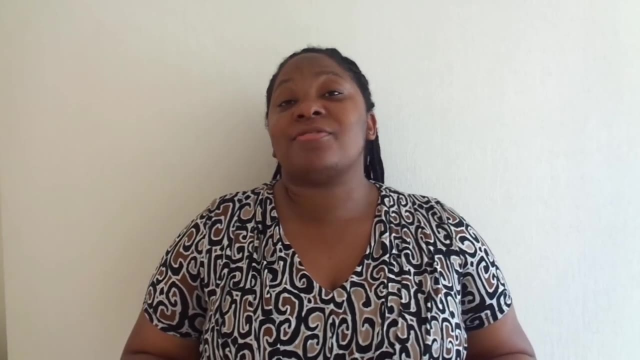 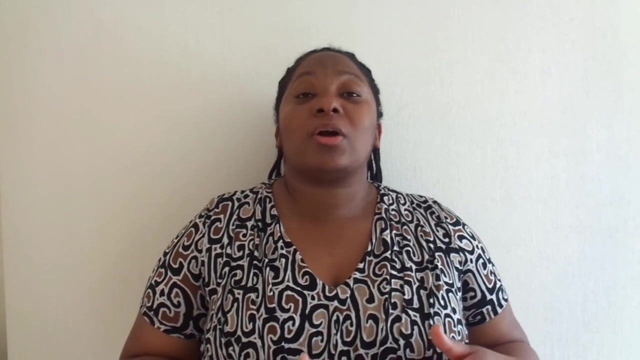 approach suitable for individuals in each developmental stage or phase. This way, the best approaches are utilized to achieve the maximum outcomes for pedagogical advancement, students' achievement and the growth of the wider learning community. Consider what kind of leader you are, your adaptability and the styles that best serve you and your learning. 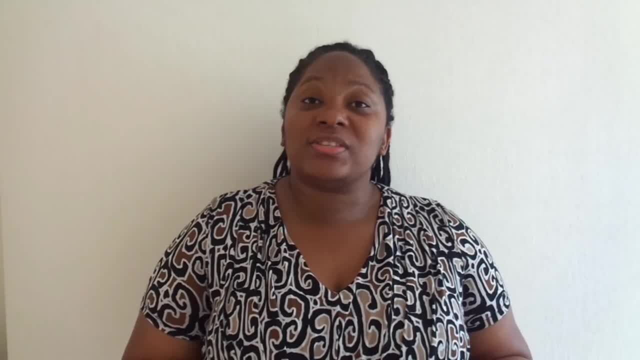 So that those can be used and implemented as best as necessary in each and every situation.